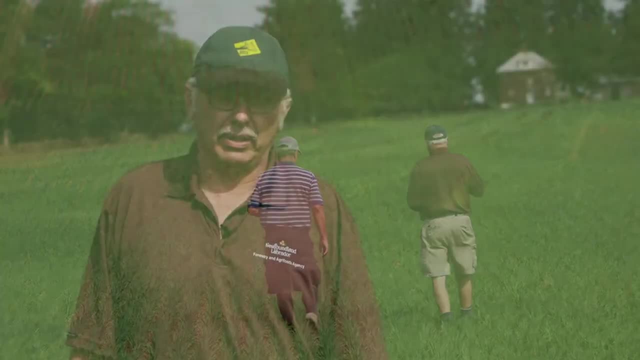 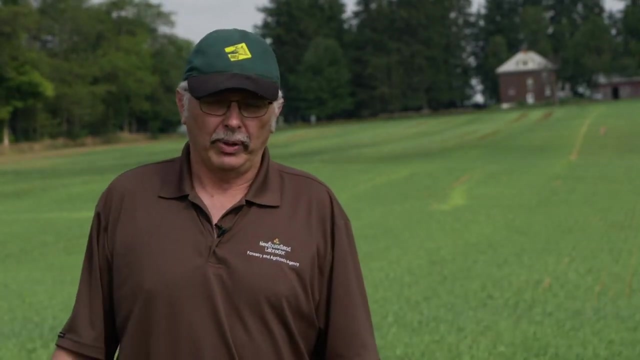 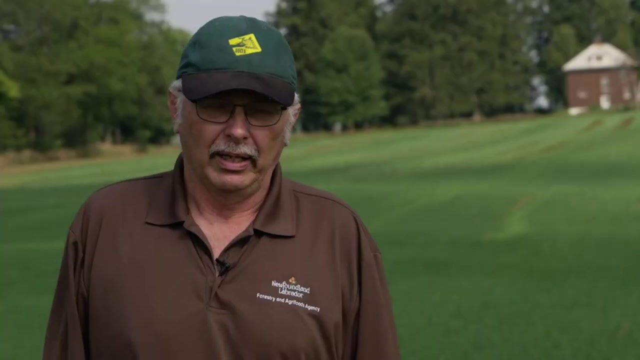 that soil in place, So we've had to put in wash cobs berms, if you like, to control the water dam, the water up. We have hickam bottoms that direct that water down into tile systems and take it off the field, where it causes a lot less damage. We do no till to leave lots of residue. 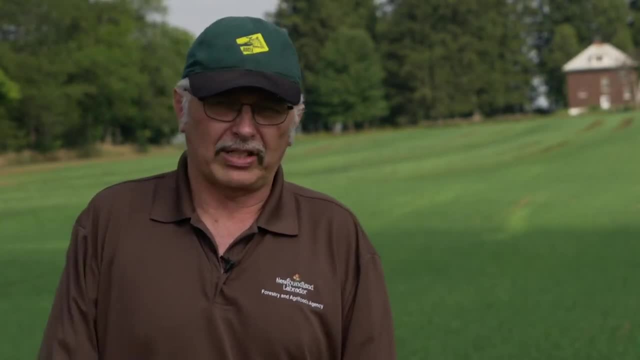 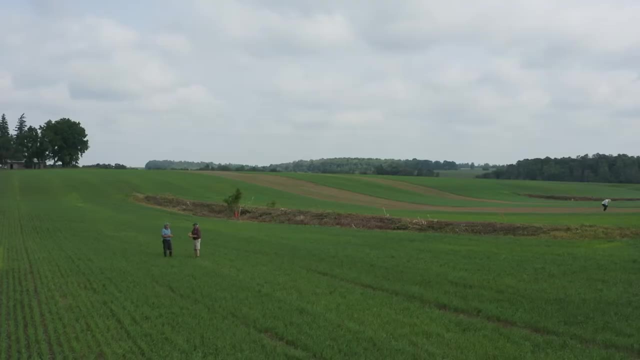 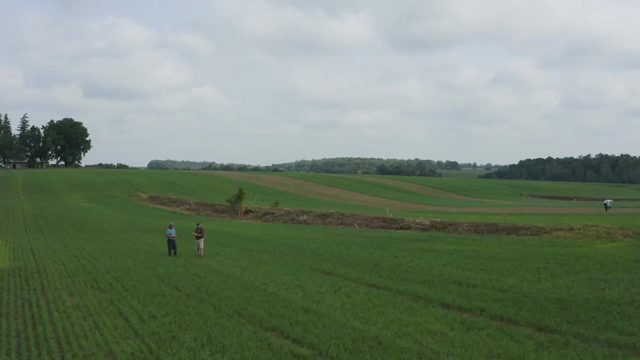 on the surface. That residue breaks down the impact of water hitting the soil but also slows the soil movement across the soil when the water is moving. And then we use cover crops in between our regular crops where we can. The roots do a lot of good in the soil and they tie the soil up so that it doesn't move as well. 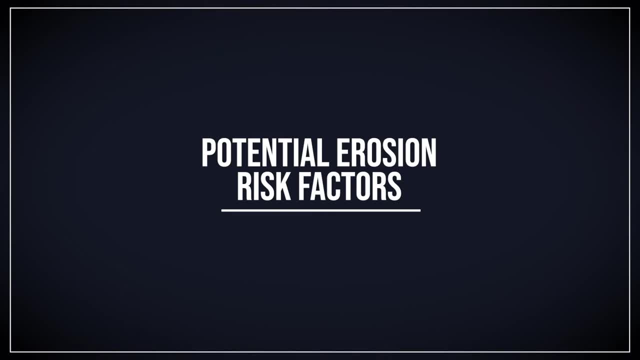 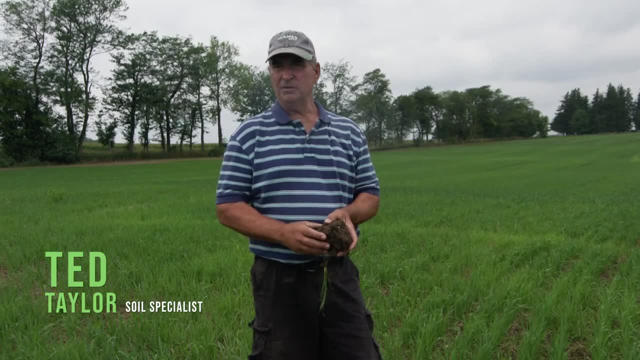 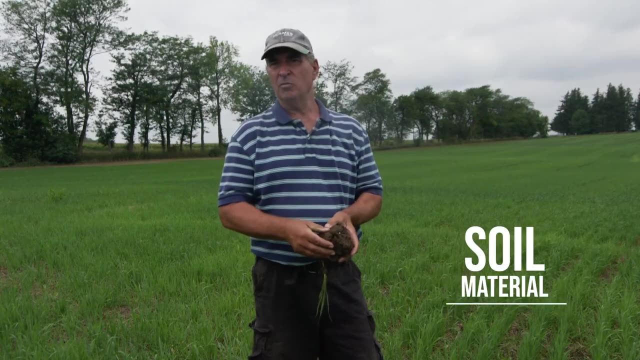 The risk of water erosion on cropland is dependent on several factors: It's the amount of and intensity of rainfall, the length and the steepness of slope. It's the soil material itself- It's more erodible than others. And it's also to do with the erosion control features. 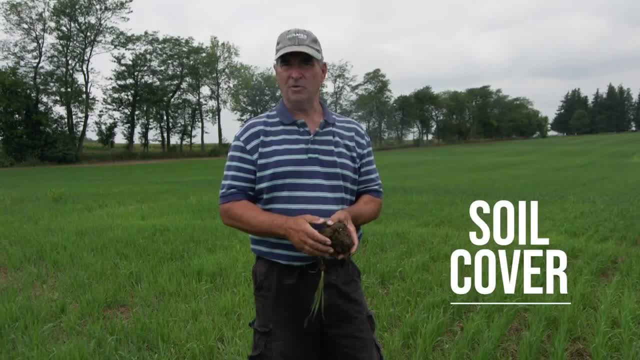 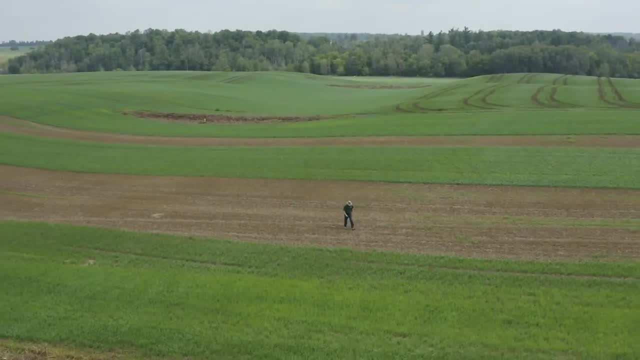 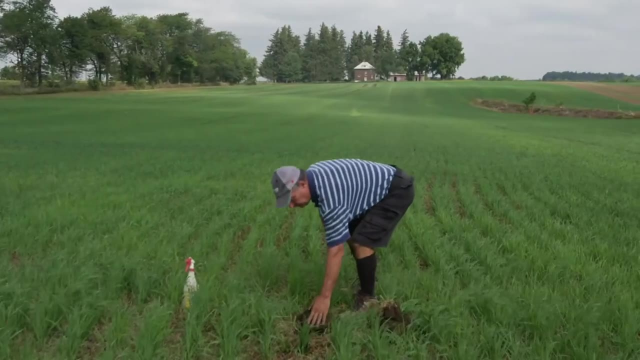 that the farmer has employed, but also on the cover, based on the crops and how much of that land is being covered. What you see here is a very long, steep slope. We're dealing with a slope that's greater than 5%. This is a very erodible landscape, So soils that are loamy or silt loams or 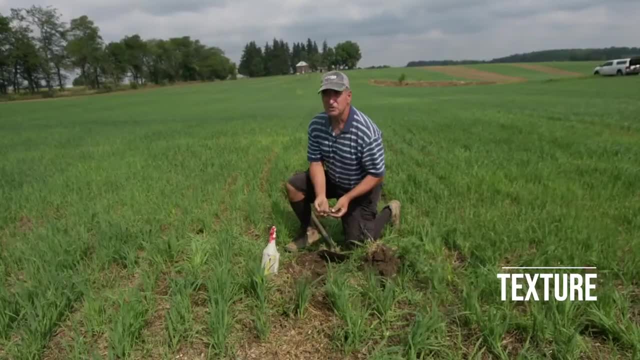 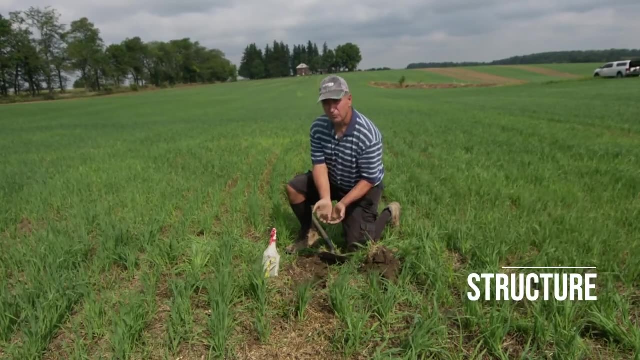 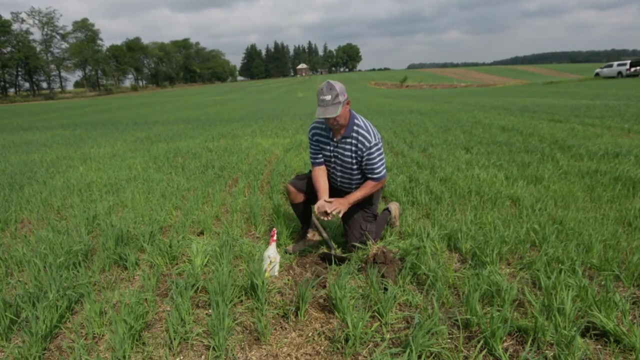 very fine sandy loams are highly erodible. Besides the nature of the soil material and the particle sizes in it, together we of course call that texture is the structure of the soil, the form of it and the strength of it. If the aggregates are quite stable, then this soil is much more resilient and resistant. 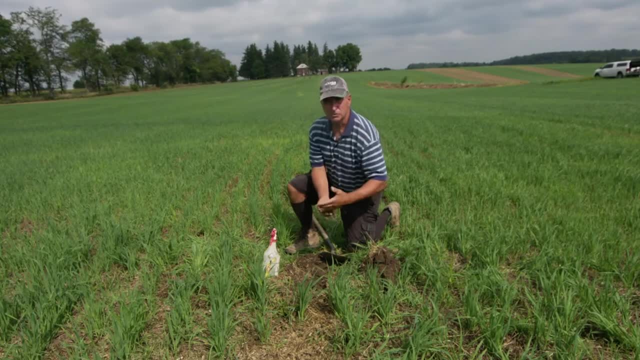 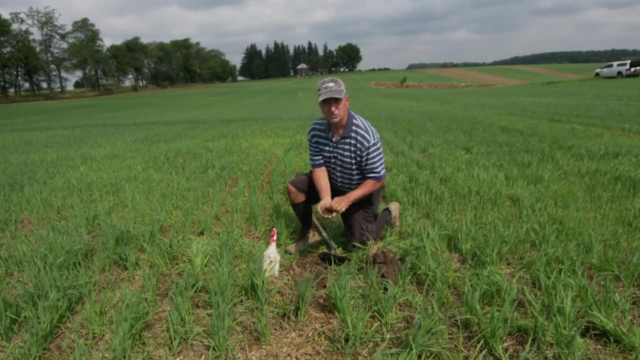 to erosion. So it's a combination of the particle sizes, which is called soil texture, and the quality of the aggregates that lead to the degree of resistance to erosion of a certain soil type. What is soil texture? What is soil texture? The soil is made up of two kinds of soil, one of which is called. 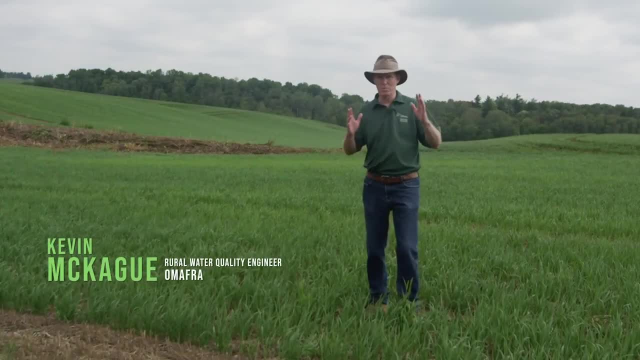 soil texture. The soil texture is a combination of soil texture and soil texture and soil texture. I'll explain that in a minute. what Gord Green's doing on this property here- I mean he's looking at it from a systems approach when he first came here. he's noticing the big cut through, this low draw down through here and 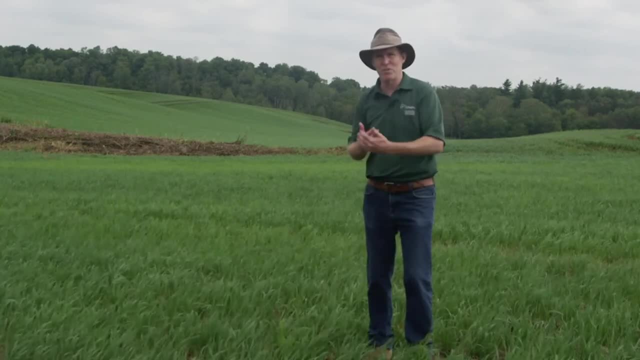 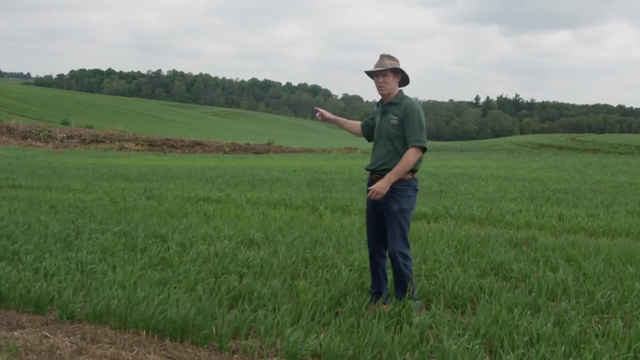 that's what most farmers generally will identify first. that's their erosion problem. they see it, it's quite obvious. he dealt with that erosion first by installing these water and sediment control basins here. as you see, there's actually three of them down this cut to sort of step that. 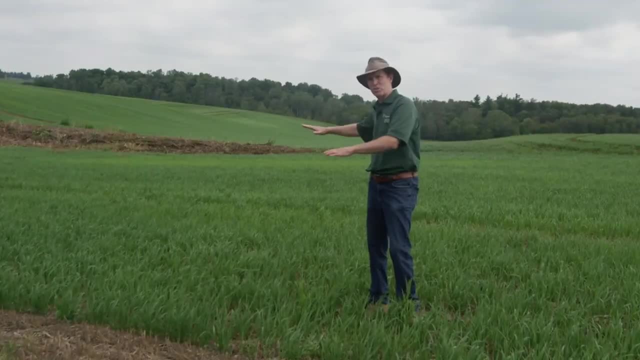 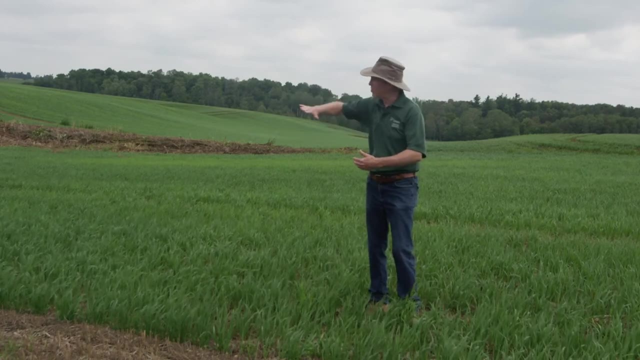 water down slowly, so that slowed down the waters is going through that low draw. but he also probably was still seeing some rilling and some sheet type erosion coming off these side slopes and it's still feeding sediment and collecting in this low, these low spots. so, moving to the 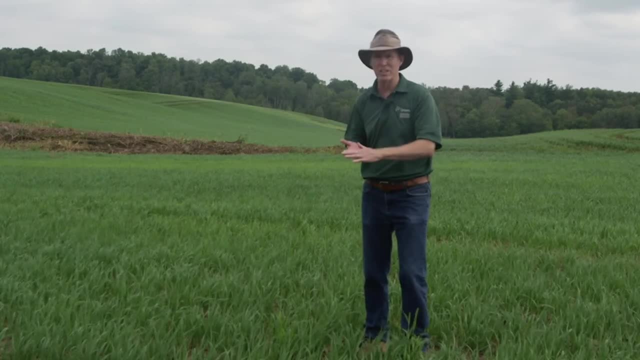 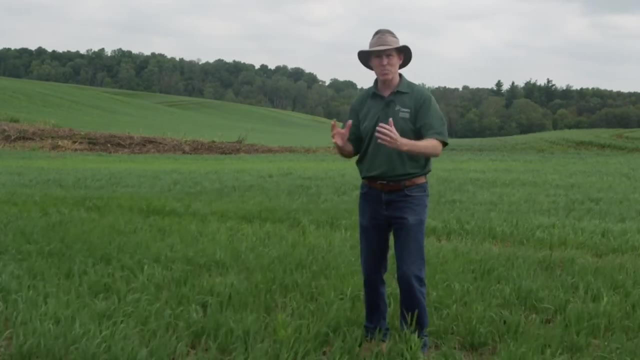 conservation. tillage, the no-till, the strip-till, and then moving into the cover crops for those roots could help to just keep that soil in place, is the package that puts it all together and so he can keep those losses down to a very sustainable rate. so 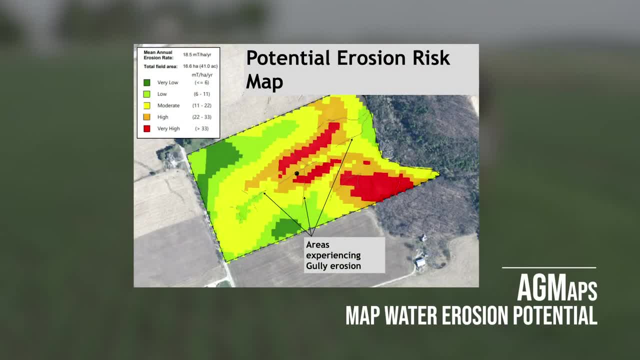 so to map, for now we have a tool that's online. it's embedded in our ag map software that you can see. you just google ag maps for Ontario and anywhere, any field in Ontario, you could map the sheet and real erosion that's in the field. so we've got a map here for this particular. 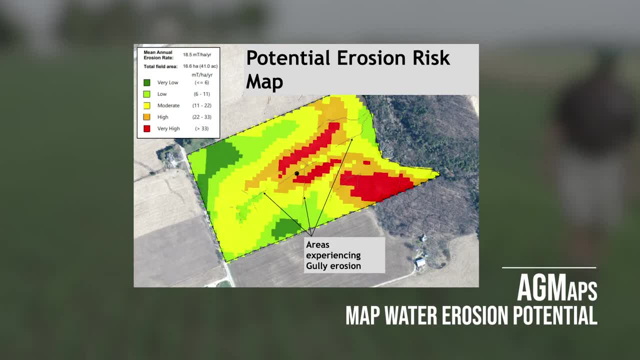 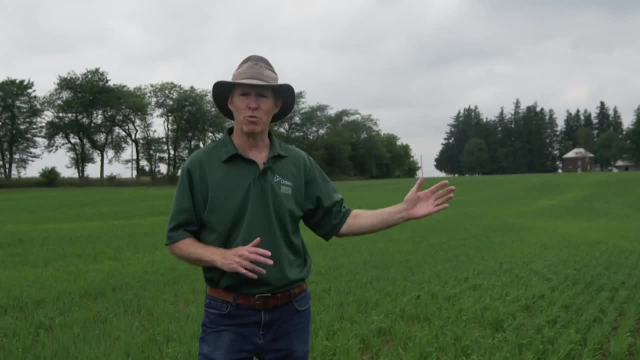 field and you can see the the areas that are more prone to sheet and real erosion. we can identify areas that are prone to gullying, and so that's where you'd want to put things like grass, waterways or water and sediment control basins, so so it gives you an ability to sort of 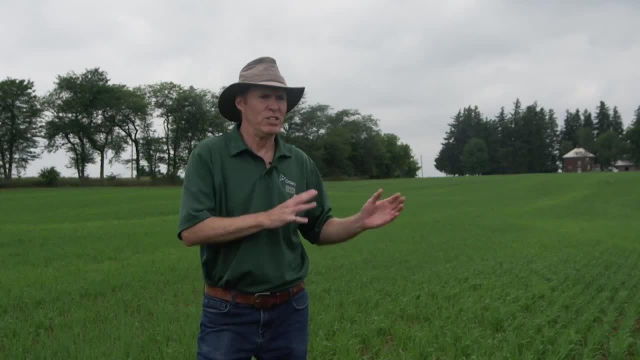 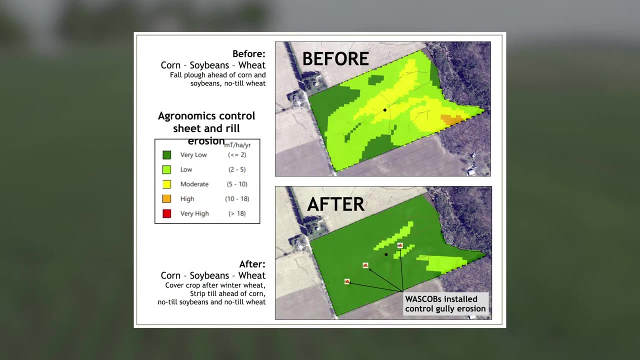 plan things out a bit better, Gord, you know he's took 15 years. started with the wascobs, looked at the agronomy. with the mapping tools today we can start to figure out: well yeah, is our agronomy going to cover a lot of this, or do we need some of these structural measures? so it gives us an ability to. 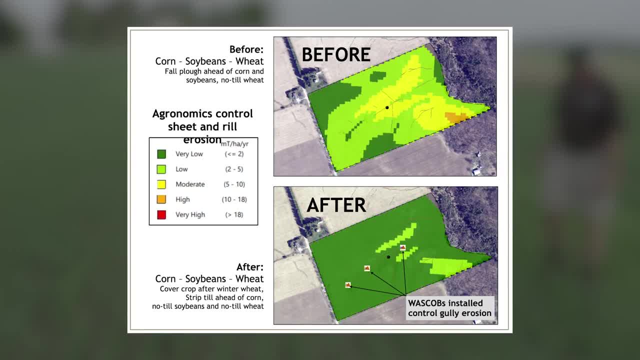 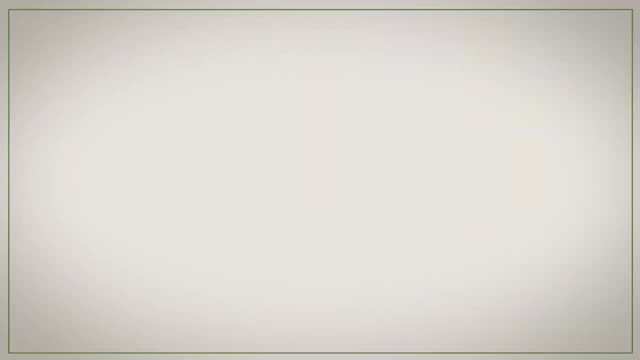 do some conservation planning on individual fields, that we may see some erosion concerns on the ag map. so that's where we're at right now. so thank you so much for joining us and we'll see you next time.